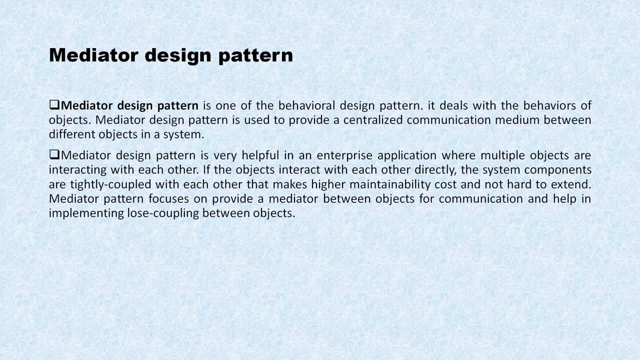 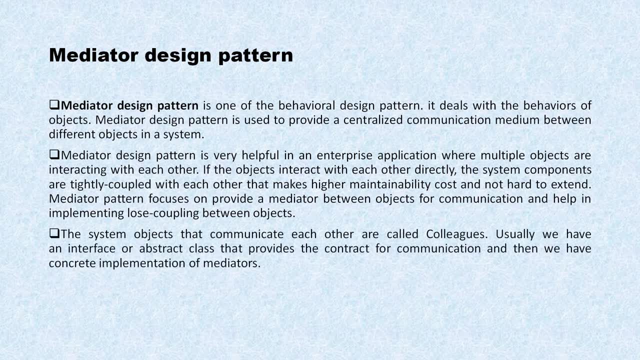 with each other or communicate with each other right in the loose couple manner. then mediator design patterns comes into the picture. yeah, the system, object that communicate each other are called colleagues. usually we have an interface or an abstract class that provides the contract for communication. then we have concrete implementation of mediator. that means first of all we'll have to 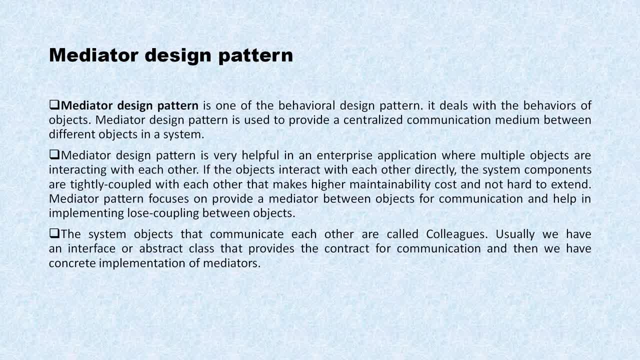 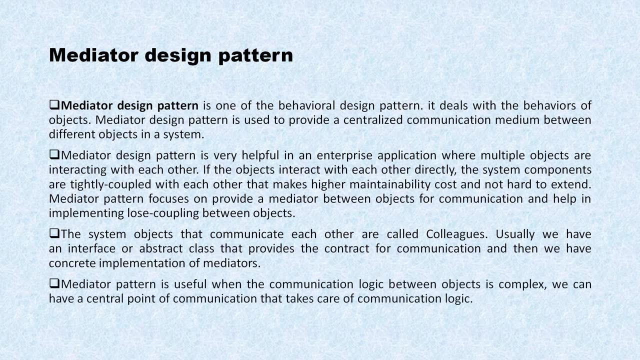 create a mediator interface or abstract class and and we have to create further its implementation and how different colleagues are going to colleagues or user is going to use this. uh, basically mediator interface, we'll see in example. mediator pattern is useful when communication logic between objects is complex. we can have a central point of 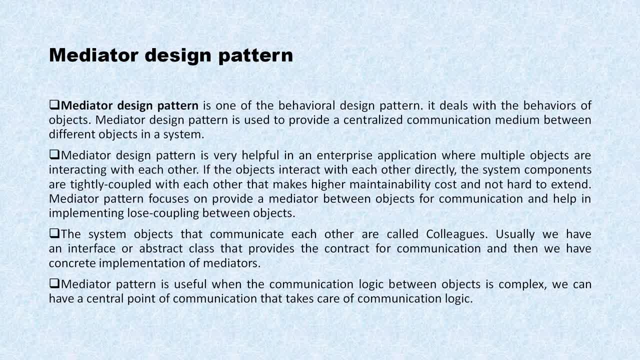 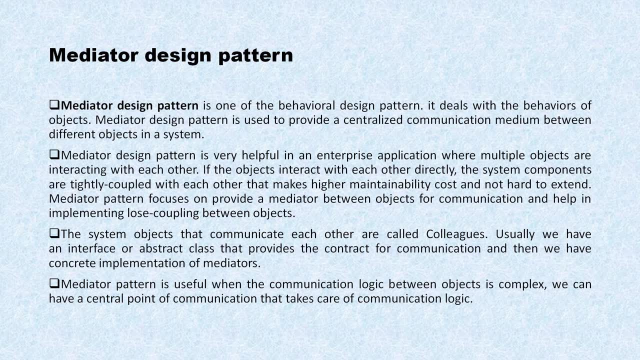 communication that takes care of communication logic. uh, there are couple of example, which is a real life example, of mediator design pattern, like, like you might have heard about, the air traffic controller is a great example of mediator design pattern where the air, air, airport or control room works as a mediator for communication between different flights. 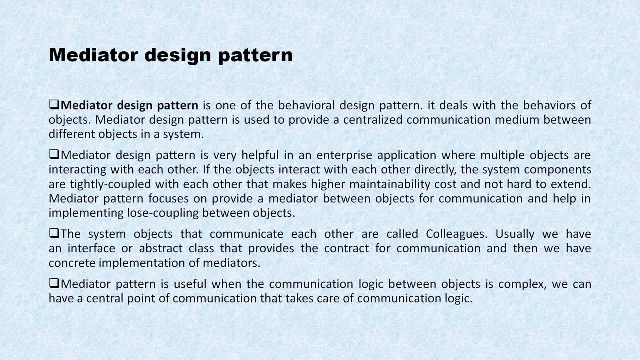 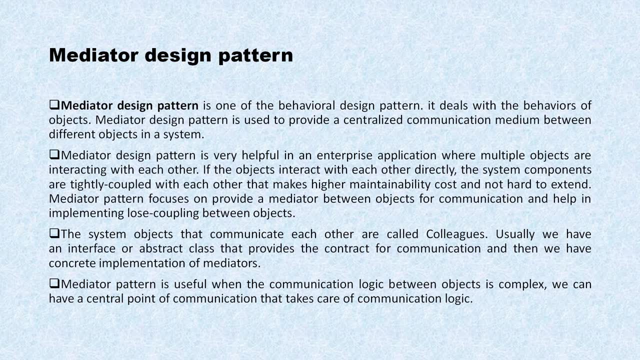 mediator works as a router between objects and it can have its own logic to provide way of communication. in this example, basically, uh will, we will uh try to implement a chat application where a user can do group chat. every user will be identified by its name and they can send and. 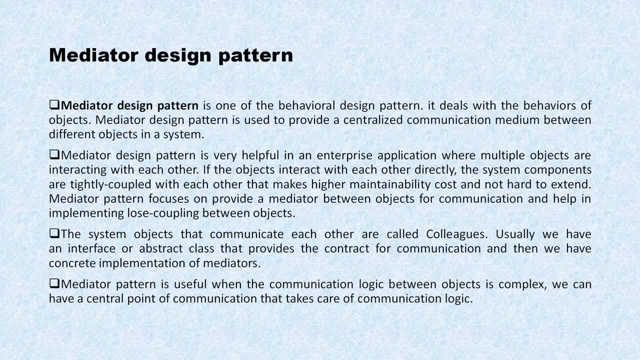 receive messages. the message sent by any user should be received by all the other users in the group that the basically use case we are going to implement. uh, in case of mediator design pattern, yeah, so here is the eclipse and here you can see i have already created a project is called mediator design pattern. 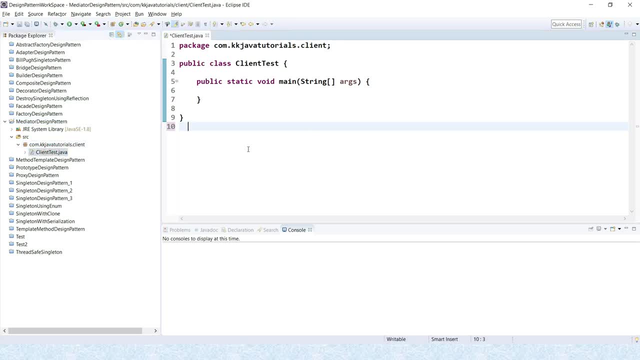 but still, i have to create a lot of classes, interfaces and after classes to implement this design pattern. right now, just i have one class is called client test, with main method, nothing else right? so let's first of all? uh, first of all, we will create a mediator interface that will define: 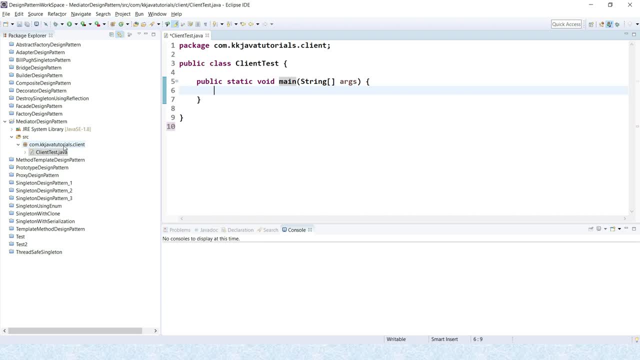 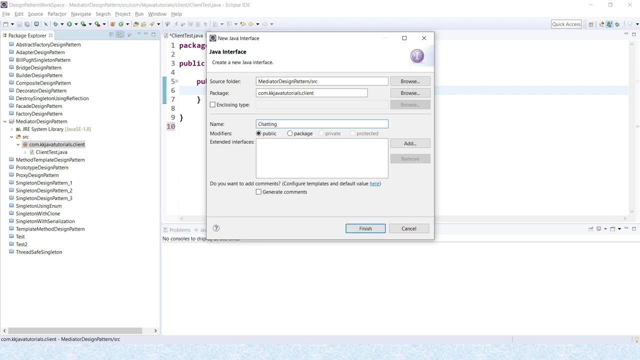 concrete or con. that will define contract for concrete mediators, right. so right, click over here, go to new, and here i am going to create an interface and that is called mediator interface. so here i am going to create chatting, or you can say: yeah, chatting, mediator, chatting, mediator interface. we are going. 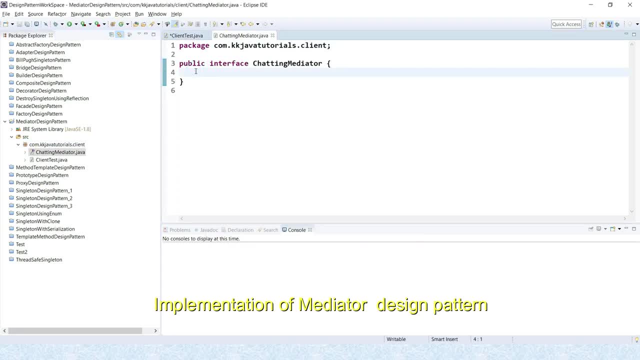 to create and in this chatting, uh mediator interface will have a couple of methods. so here, first of all, i am going to add a method is called send message, so i would say: public extract word, send message. yeah, and this will have, uh, first of all message as an argument, which is just an string, and then our second parameter, i'm going to pass a. 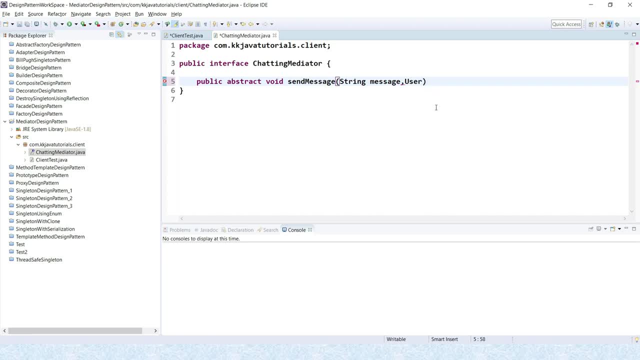 user. so user is still i. i haven't created that, i will create. so user: nobody. now second method: i'm going to add add users. right, so i would say add user and again user will have an input, so that using this mediator interface, we can add a user in the group as much as user we want to add. 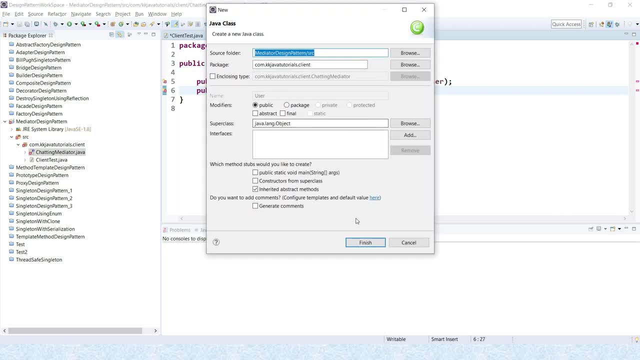 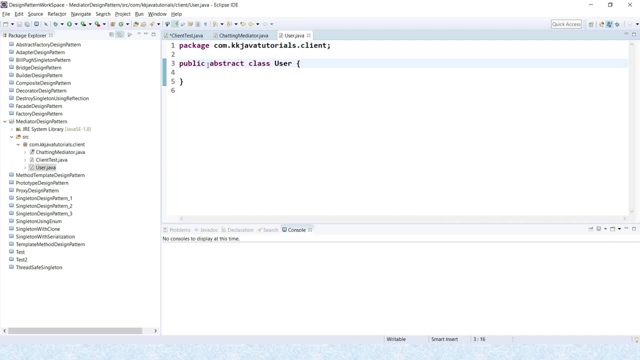 right now we need to create a class. it's called user, and this class i'm going to keep as abstract class. right, so we have a user class, so this class can be considered as a mediator pattern colleague. right, so this can be an interface, or you can, uh, write a abstract class as well, right? 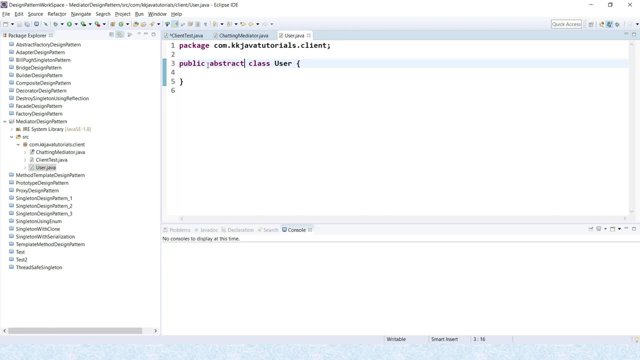 so user can send and receive message, so we can have user interface or abstract class. so here i have created user as an abstract class, right, and this class will have a reference of mediator. so here i'm going to provide a reference of chatting mediator right: directing mediator. 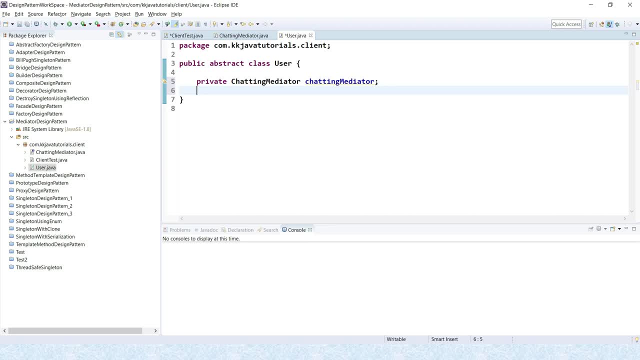 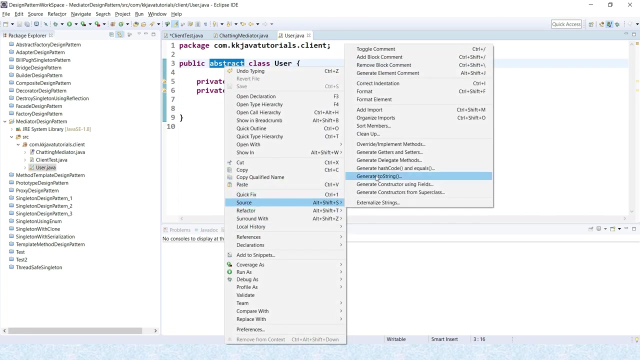 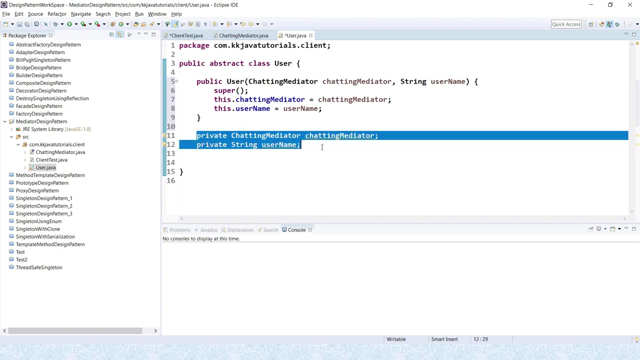 and of course, uh, we want to identify each user by its name. so, second variable: i'm going to declare as username here and as we this: this is just after class. we can of course create a constructor, so i'm going to create a construct out of these fields. and second thing: sorry, uh, this property i want in the. 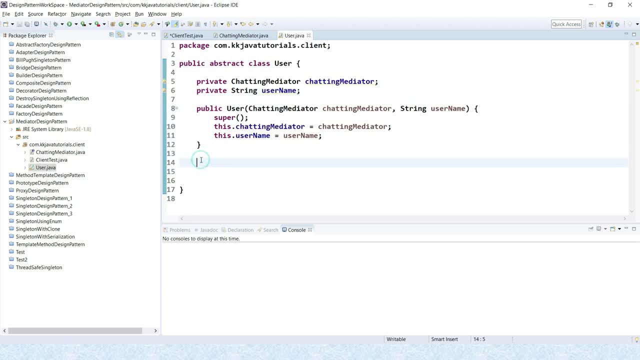 beginning of the class. and second thing, i'm going to create a public gator for this uh reference for this instance variable. so create a gator. so just, i'm going to create only gator for this. okay, now couple of abstract method i'm going to add over here. first method i'm going to add send message and then receive message. 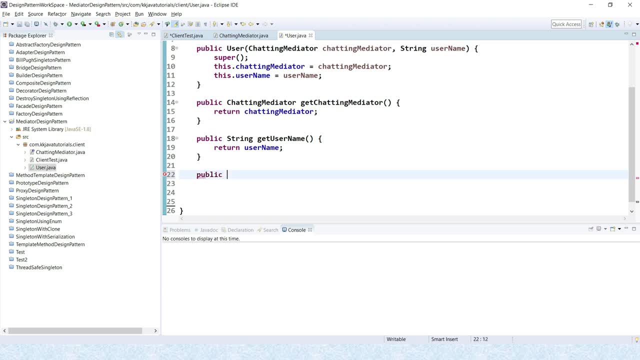 public, public abstract. so of course, this method i'm going to add as a as an abstract method- public abstract word- and i would say send message. yeah, send message will have only one parameter is called message, and then we'll have a receive message. and second abstract method i'm going to add receive message. sorry, 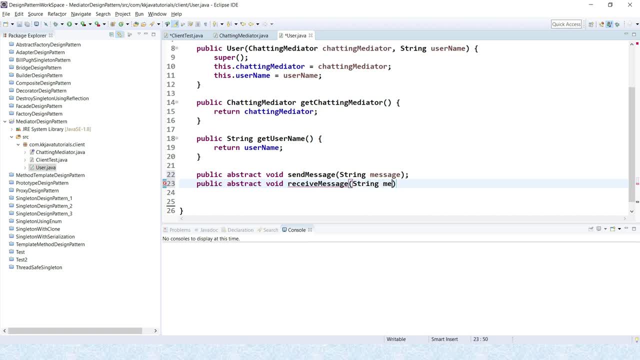 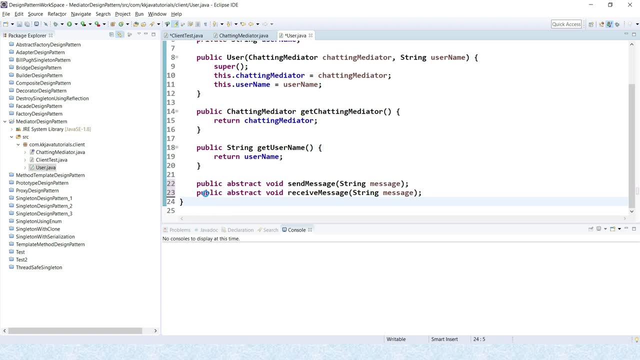 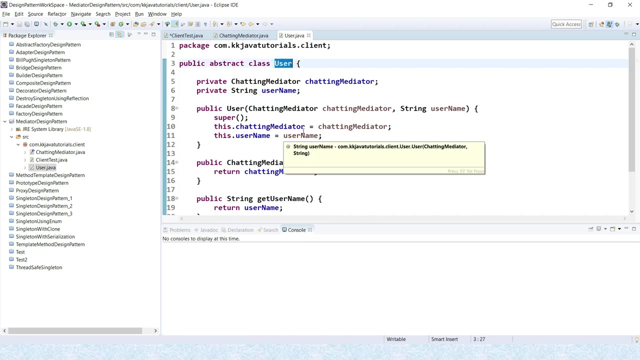 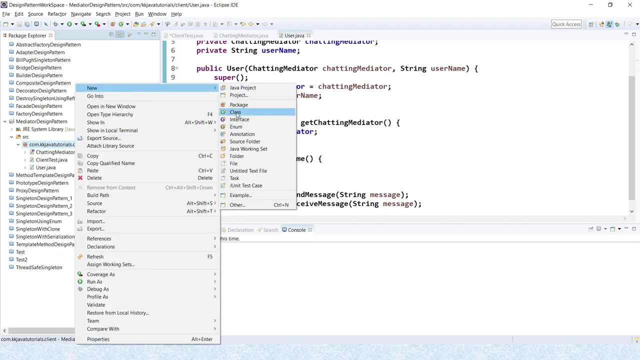 receive message and this will have again string as an argument, that is, message which is going to receive by the user. yeah, that's it. so we have defined- uh, colleague, or you can say, user abstract class. so next i am going to define most of the things i am going to done with the same package. afterwards i will re-energy it into different package. 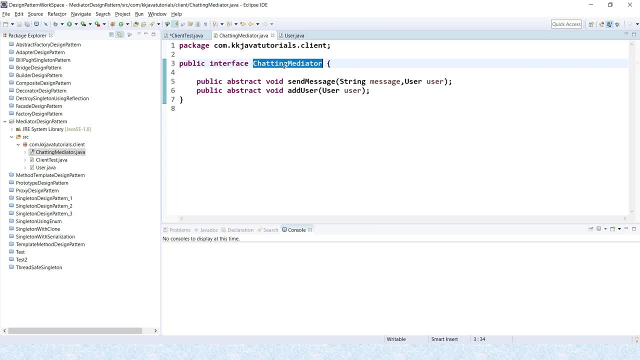 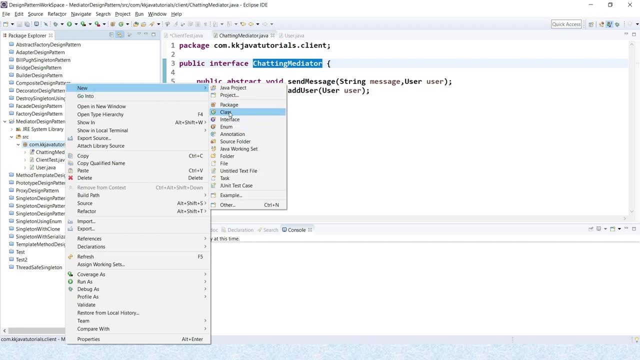 now i am going to create implementation of this guy, right, implementation of this mediator. so right, click over here. then i will say class. class name would be chatting mediator impl, and this is the class name and this is chating mediator: imp will be in chatting mediator. next, i'm going to write right and write mplu, and i'm going to write chating medial- chating mediator, and this is the chatting mediator ability. so right, click over here. then i say class name will be chatting mediation, j wurden. i'm going to writelike this и пойдly steering class: О dailyacağ у вас parl. 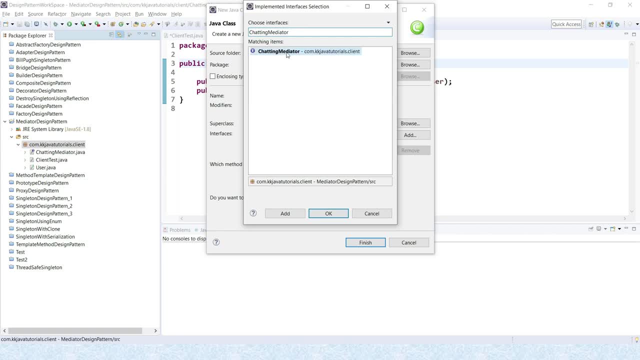 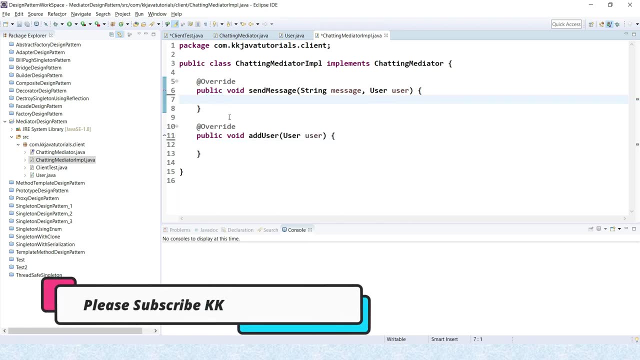 guy is going to implement chatting mediator interface, right? so this is nothing but a chatting mediator. so chatting, or chatting mediator or implementation class will have a list of users. so here I'm going to create private list of user. yeah, yeah, I would say user list. okay, just import. 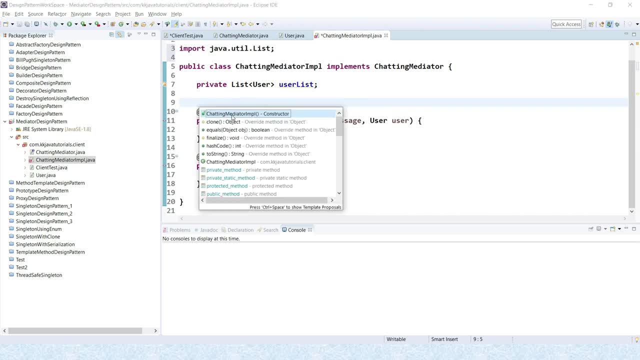 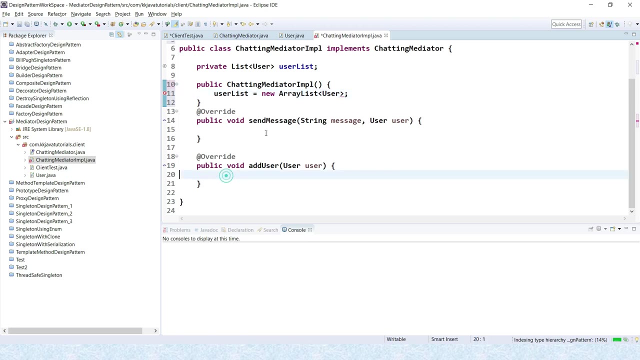 the order and here I'm going to create a constructor. so- and here I'm going to initialize this guy new�시aruelist. yeah, cool, now we have added here. so in this user list, user- I mean client- should be able to add multipleelists. so I'm calling this. 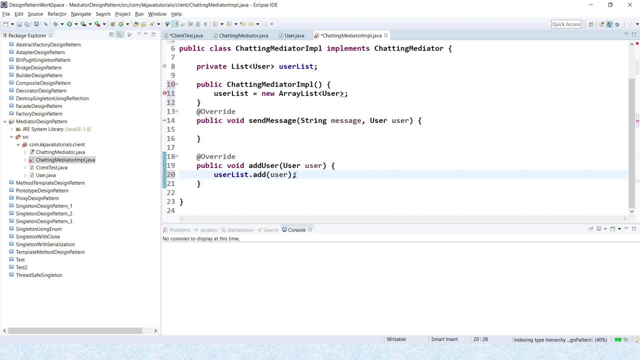 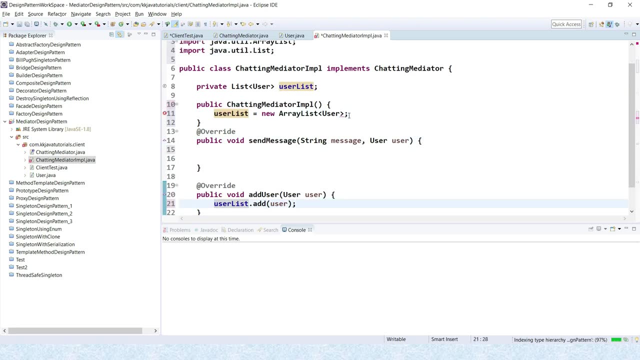 method. yeah, now we have a method is called sendMessage, right, so here sendmessage, as we have a list of users here now, sorry, so here we are going to put lately of users. yeah, now, list of users we are iterating over here, so this two variable name is same. that's why this guy is throwing an error. so let's say this is: 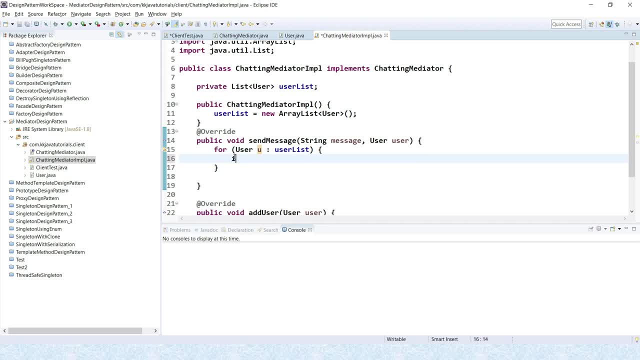 you now inside that what we want. here I'm going to write some code like you: dot gate username right. dot equal ignore case: this user don't get name, get name. and here I'm going to write a condition: these two user names should not be seen. so here what condition I'm going to put. message should not be a received received. 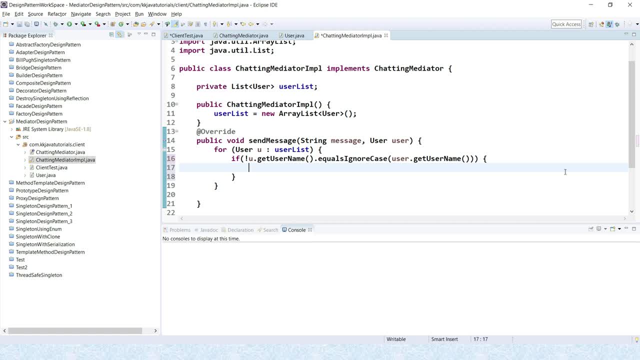 by the sending user. right. so user who is sending the message should not get the message back, and after that I'll do so for every user we want to send the message, right? so user dot. I would say the received message. same message user will receive. but user who is sending the message that should not receive the. 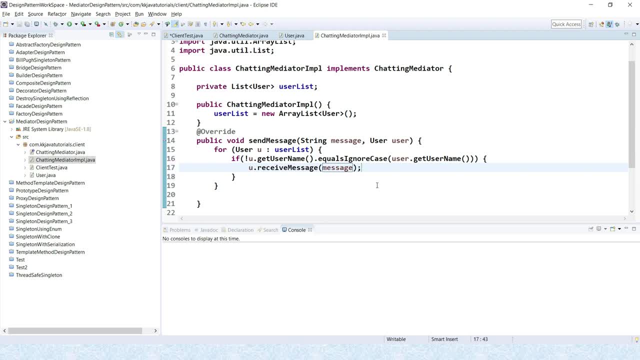 same message back. that's the condition i have given over here, yeah now. so we are almost done with the uh, this guy right here. one thing i would like to do so here: we have added user list right, and we have a list of user they that we have any slides over here and user can uh, basically. 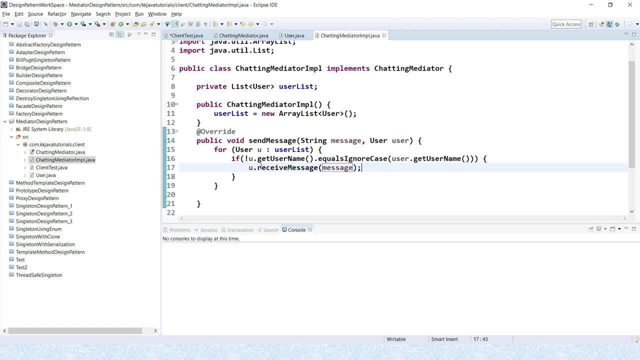 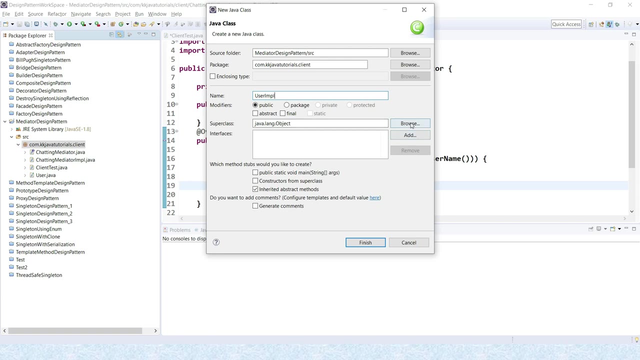 send message to the. every user in the group except user who is the sending the message itself should not get the message back. now i am going to uh create a user impl, user impl class and that basically extend. a class is called user right. this is nothing but a colleague. 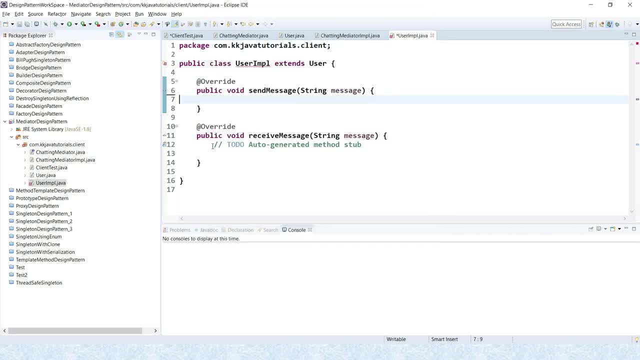 right in the case of mediator design pattern. right, and here, uh, there is a constructor in this class, right, which, basically accepting a chatting mediator and username as an argument, right, so we have to, uh, basically, we have to, uh, basically, uh, send this as an argument, as a super right. 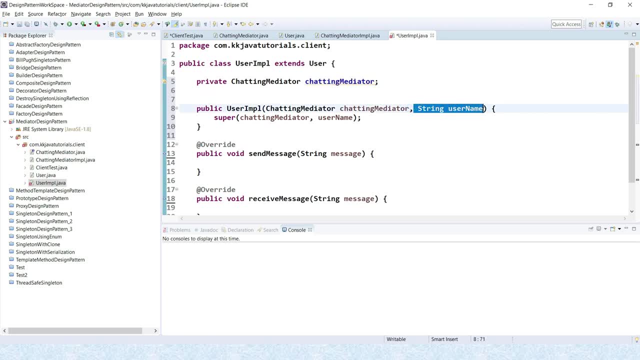 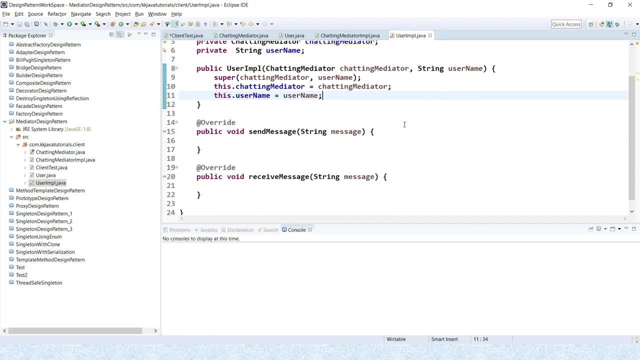 and here these two i am going to declare as a private variable private user. right, and here what you can do: this dot chatting mediator goes to chatting mediator here and i would say: this dot username equal to username, cool. now in this user impl. uh, we have to. 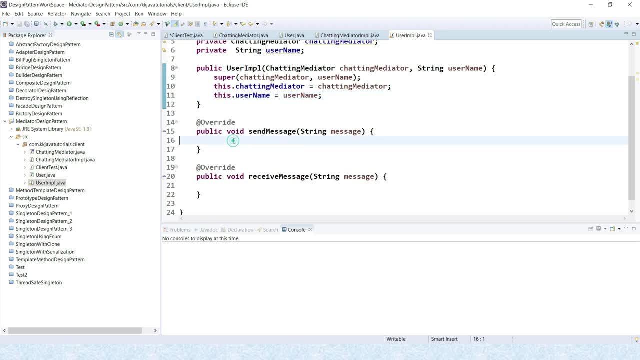 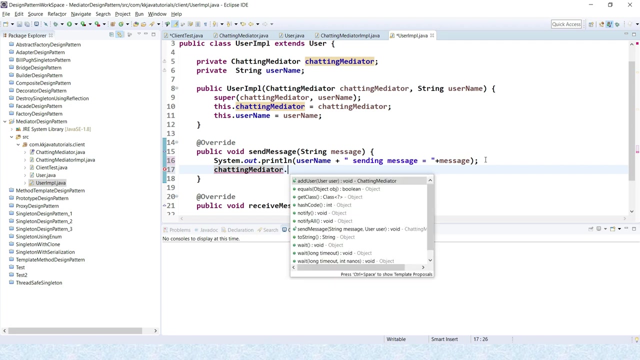 overwrite to miss method right first: send message method. send message method. so here i am going to write a message. uh, here username that's a sending message equal to message. cool, now we have a reference of chatting mediator that we can make it make use over here. here i'll say: send a message. 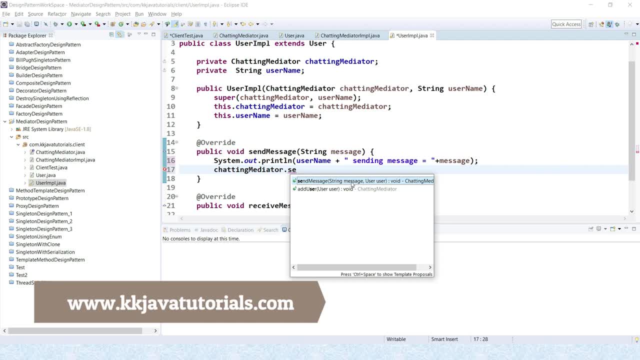 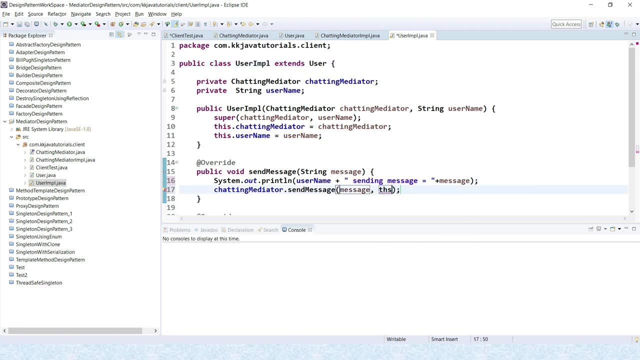 right, so send message. taking two argument: one is the message, that is a string which is already coming from uh, this method itself, and second is a user. so user. here you can say: this guy is basically extending this user class, so current class reference variable. this we can send it okay. 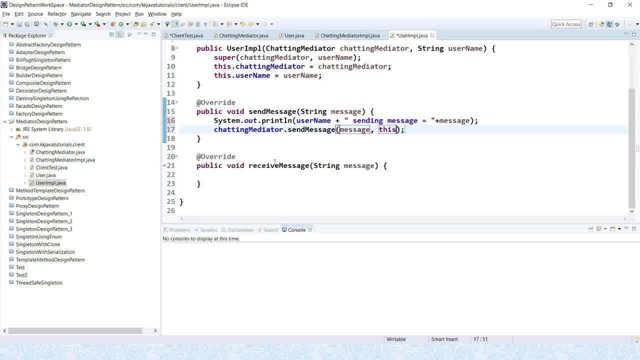 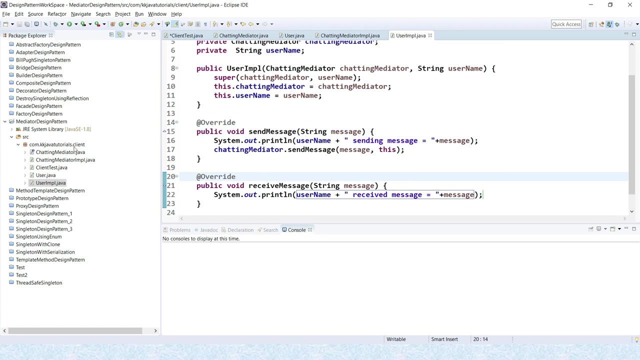 right now we have a received message, so every user should receive a message except a user who is sending message. so i'd say user name: received, received message. message equal to this message. cool, now we are done the implementation of uh user as well. right now we have a client program here. so what we can do, we can do some. 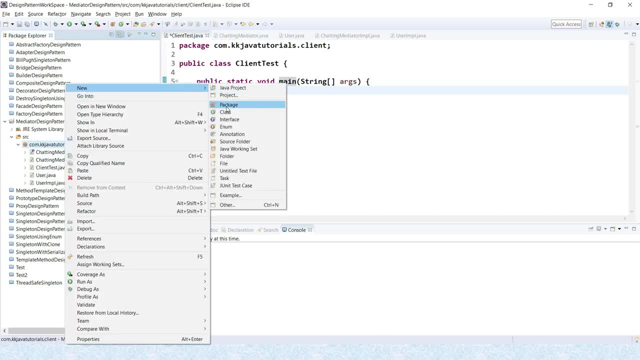 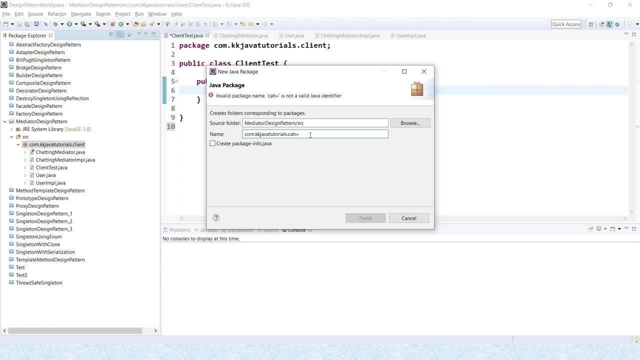 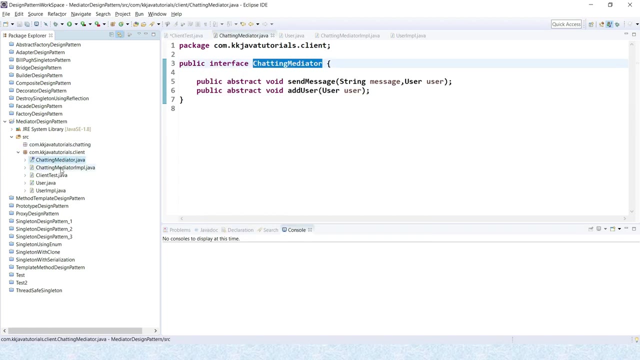 kind of refactoring, right. so here i'll go to: i'll create a new pack package. i'll create a chatting, chatting package and all the classes except except client program. i'm going to move it over here in this chatting package. yeah, i moved here. okay, now in client program, what we can do. 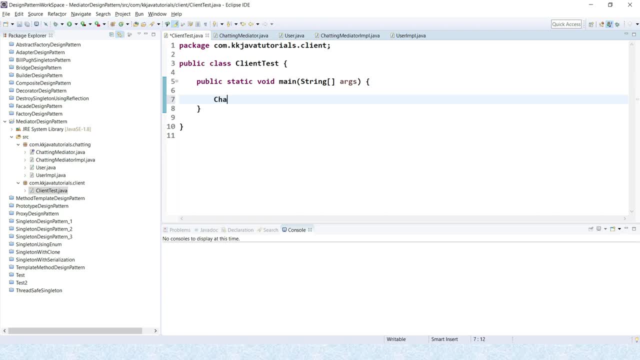 client program. i'm going to move it in this chatting package. okay, now in client program, what we can do. we have to create a chat, have to create a first of all chatting mediator, object setting mediator. so this is an interface. you cannot create an object of this interface, but you can. 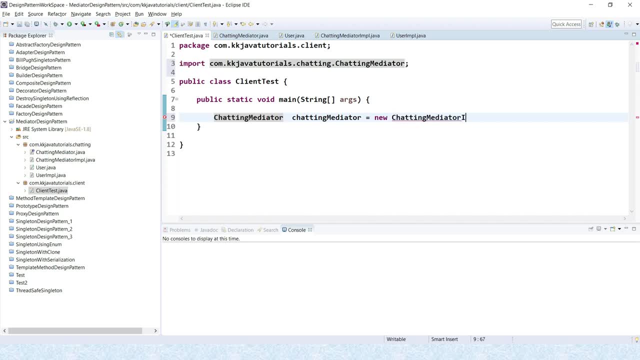 create an object of its implementation I can assign to this reference. yeah, so I have created our chatting mediator reference and now we have to create few users. so I would say user. let's say: this is user one culture, new user. I am so sorry. so, user, we have a user. I am peel right, so we can create an object, this. 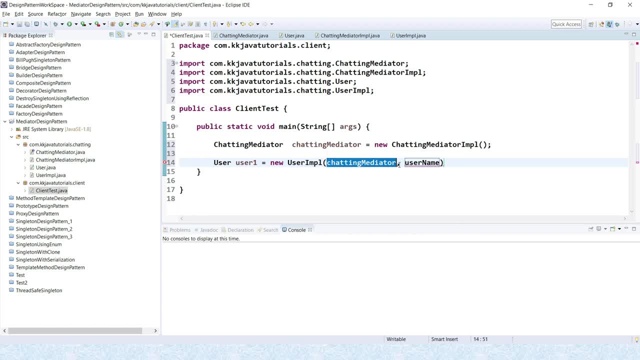 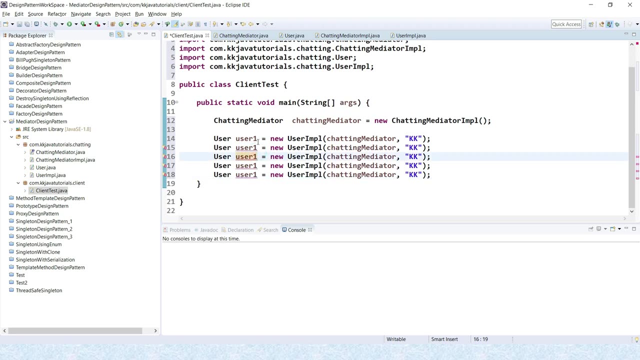 guy is taking first chatting, basically chatting, mediator reference. second is the user name series, or I'm going to specify KK, so just I'm going to create few users. let's say I'm going to create five users. five users have created here, and this is user two, then user three, user four and 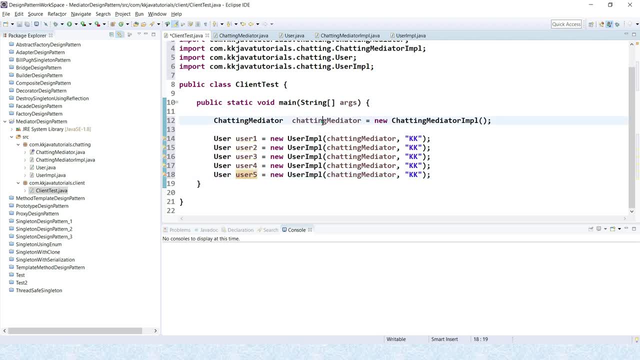 user five: yeah, now in this chatting mediator we have to add these users, right, so here let's change the username as well: KK, PK, MK, SK, VK. yeah, just simplicity, I have used given the username into letters. right now chatting mediator has an ad user method, right, so we have to add these users. so user two: user one: I have added. 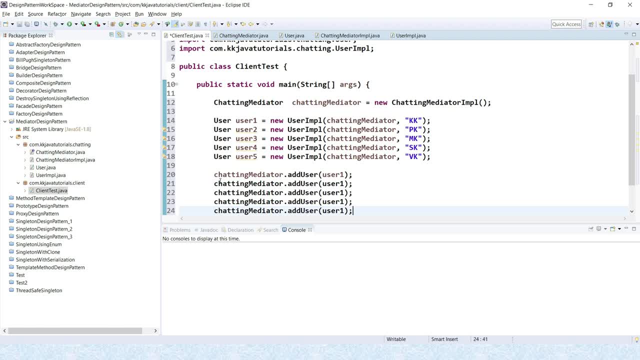 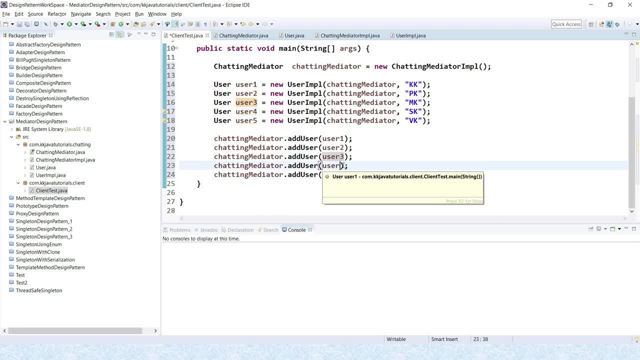 user one, then we'll cut all these users in this chatting mediator. so usually one is your two, user three, user four and user five. yeah, now let's say user to, which is PK, is sending message to the all the users. so user to dot I, it's a. 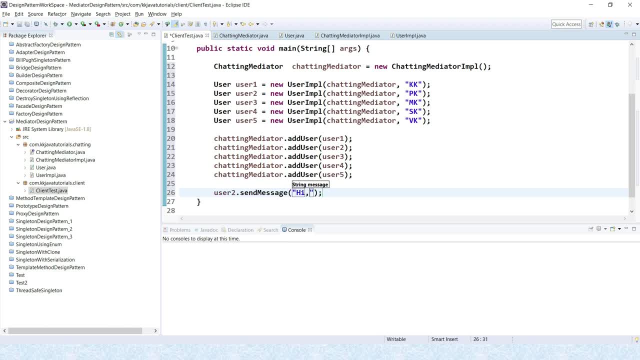 same message here. user to consent: hi all, yeah, to all users. so this message should be received by the user one, three, four and five, but should not receive back by the user to itself. right, so let's run this application and see how this application works. so here you can see. PK means the user to has sent message to. 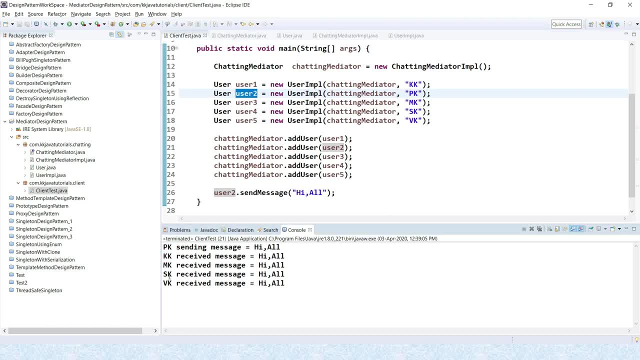 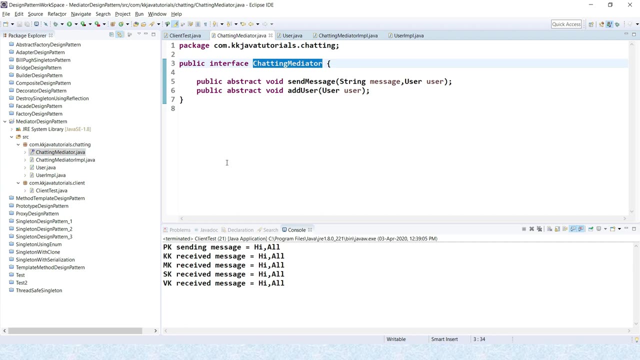 all the users in this group- this of these are like KK, in case can PK- are receiving the same message. so, guys, this is the perfect example of mediator design pattern, so let me, let me explain each and every files again. so here, first of all, we have created a mediator interface and media chat that is a 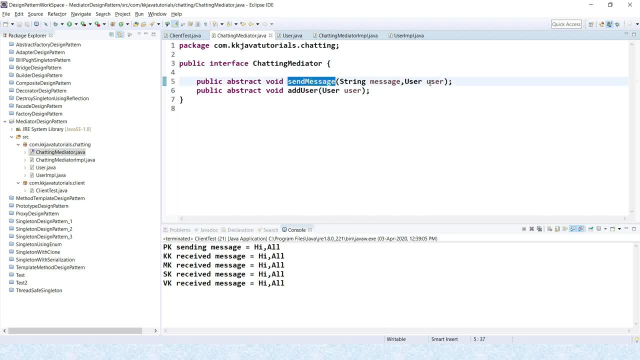 static mediator and which will have a two methods: send message, sending message directly to the user. so this is the perfect example of mediator design pattern to the user. so we have a message and user as an argument and add user right. so as much as user you want, you can add in this group you using chatting mediator. 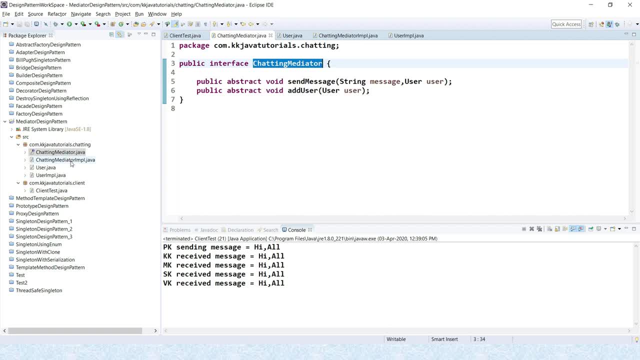 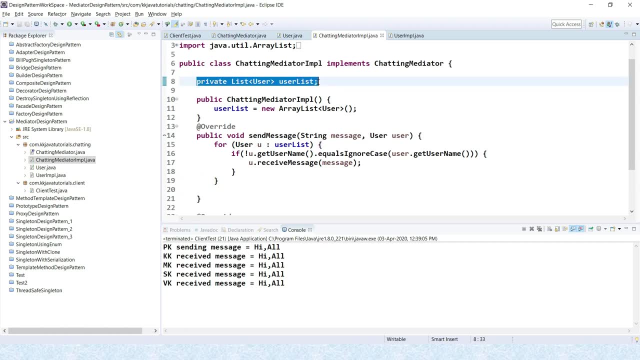 right. so of course we required is implementation. right, so that's what we have created: chatting mediator implementation, which will have a list of users, right so? list of users we have declared and same. we have instantiation, instantiating within the constructor. so when a client will create an object of chatting mediator, IMPL, this will be. 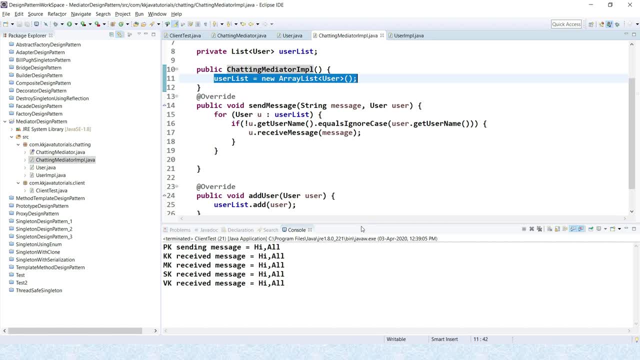 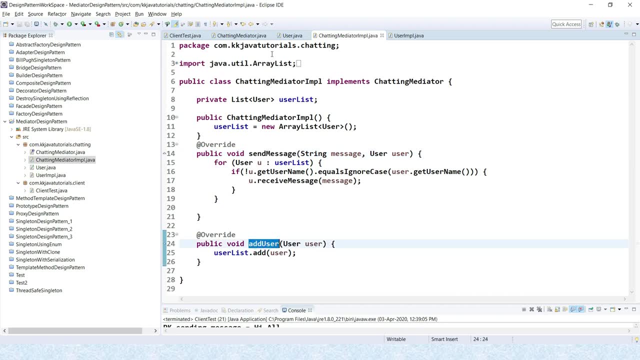 automatically instantiated. yeah, and this mediator implementation class will have a method- is called send message and add user. right, because this interface is having two methods. so this is the responsibility of implementation implementor to implement these two method definition right. here we are iterating list of user and make sure that user who is 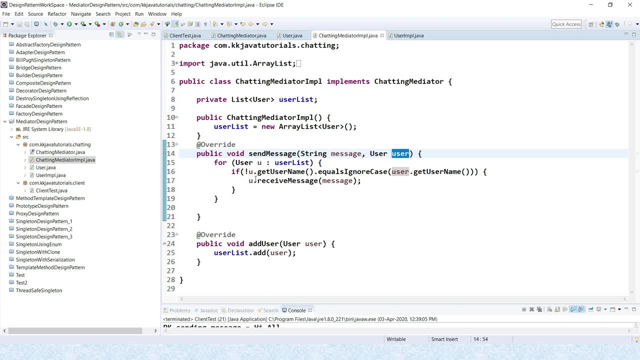 sending the message should not get the message back. rest of the user should get this message. so we are taking each user from this list and sending this message which is coming from the sender. right now we have an add users to add users in this list. pretty simple. then we have a user which. 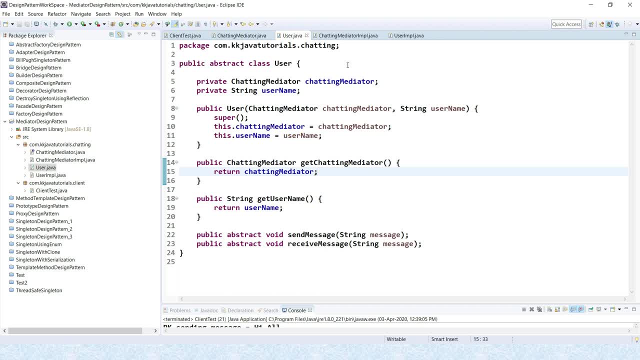 is which is considered as a basically colleague in case of mediator. design pattern, right. so user has a reference of chatting mediator and user has a name so that we can identify the user. now we have a constructor which accepts chatting mediator and username, right and just. we have initialized over here and we have provided a public setter getter method by 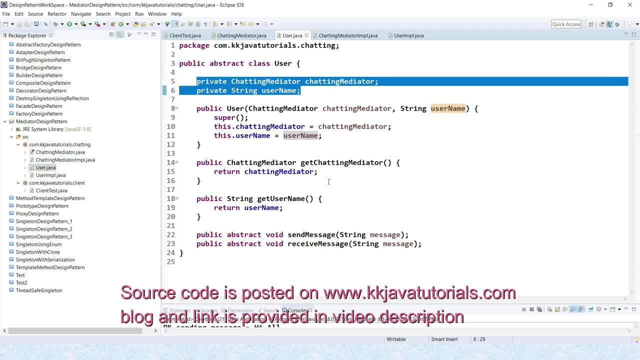 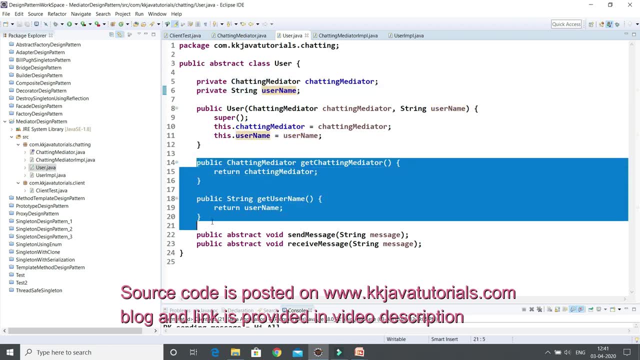 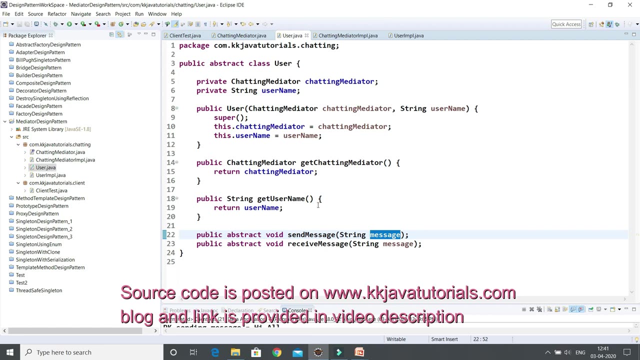 making this variable as private right. so whenever we have to basically try to access the reference of mediator or username directly, we can call by getter method. and we have two methods: send message and receive message, which is accepting message and argument right, and we required subclass of this guy. 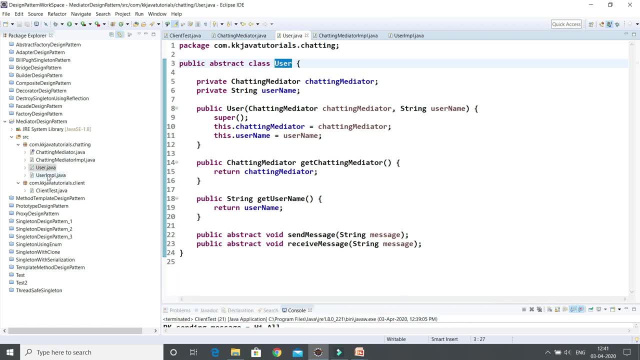 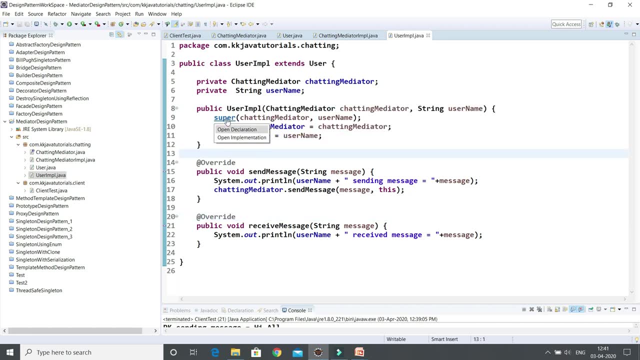 because this is a just an abstract class right. so that's what we have: a user IMP- I have given the name which will have again constructor, which will call this superclass constructor, by bypassing reference of chatting mediator and username right and same I have declared here and initialized over here. so here of 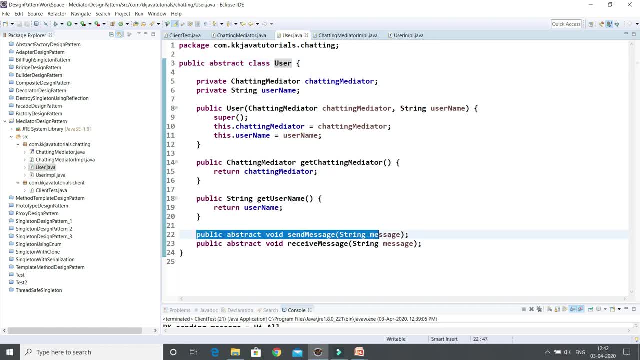 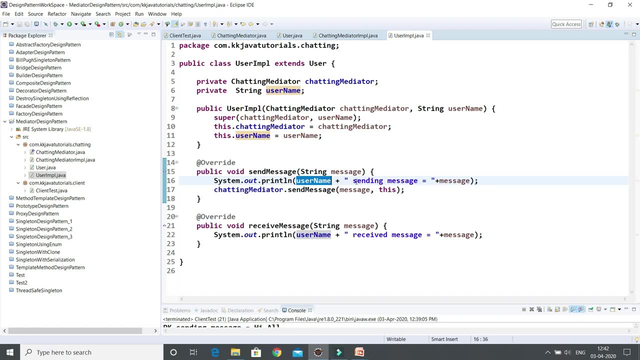 course this user abstract class is having a two abstract methods, so these two method has to implement by the user. I MP and that's what we have done. so here, just we are printing a message, whoever user is sending message that so that username and message is getting. 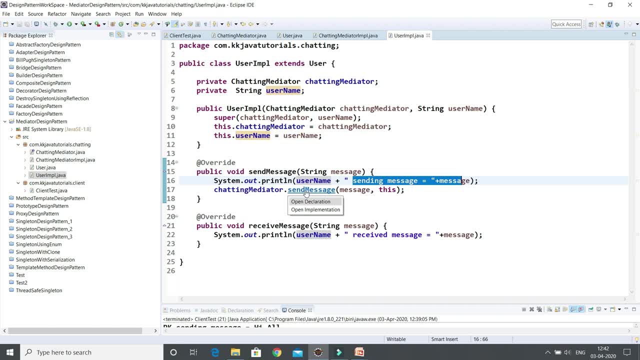 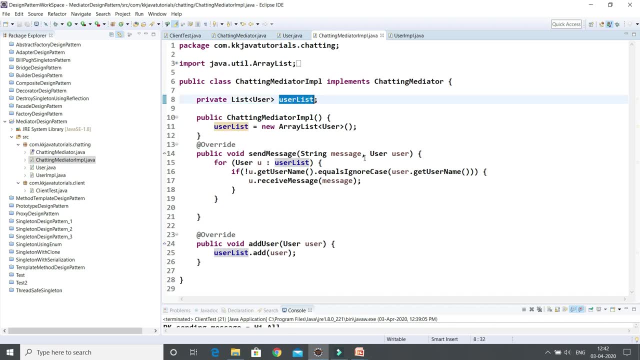 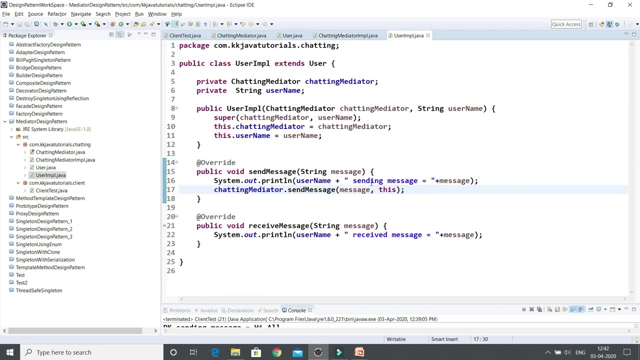 printed over here and within that, just, we are calling send message, right, so send message will call this guy and all the users. I believe, in the list of users we have a list of users in the group and for every user we are sending this message, right, cool. and now we have a received message which is basically: 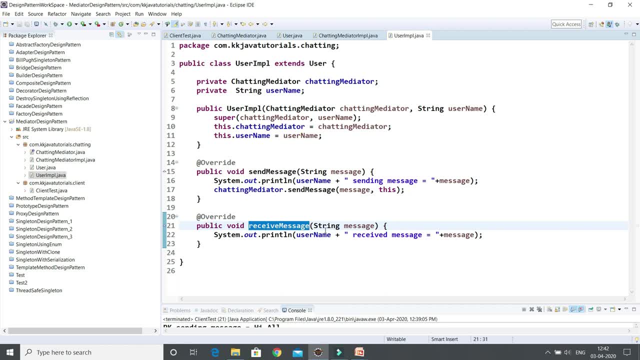 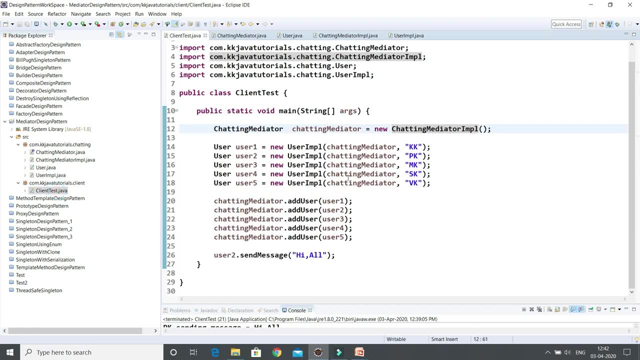 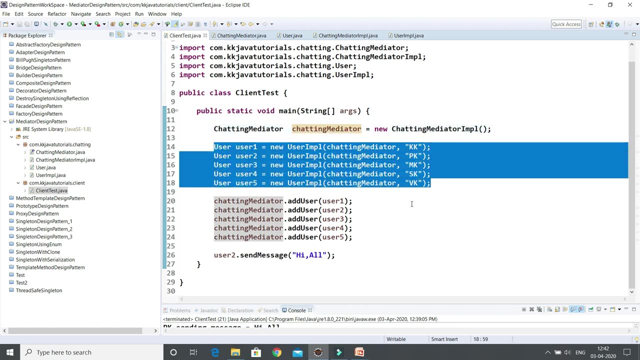 just getting called by the. every user who is receiving the message and user name and corresponding message is getting printed right now in client program. we have created a chatting mediator and we have created of five users. we have added all these users in this, in this, in this list, right? so if